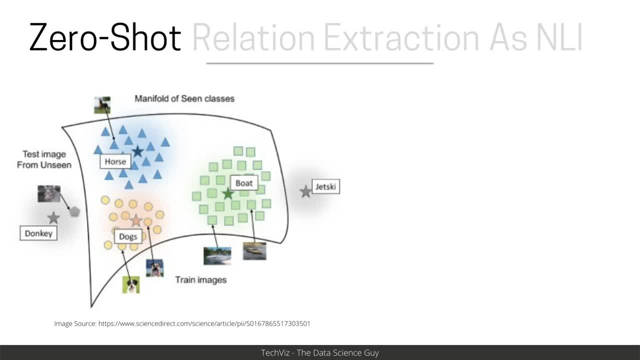 is the example of ZSL. So, for example, if we have a model that was trained on image classification task on horses, dogs and boats images, Now during the testing phase it is given images of jet ski and donkey to make the correct prediction. So the idea of ZSL is more or less. 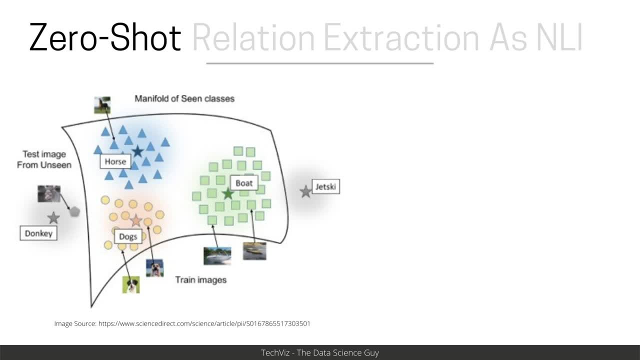 similar to how we humans also extrapolate our learnings to a new concept based on existing knowledge that we gather over time. So here there could be some common features that are shared between dogs and donkey, horses and donkey. So, based on those aspects and representations, 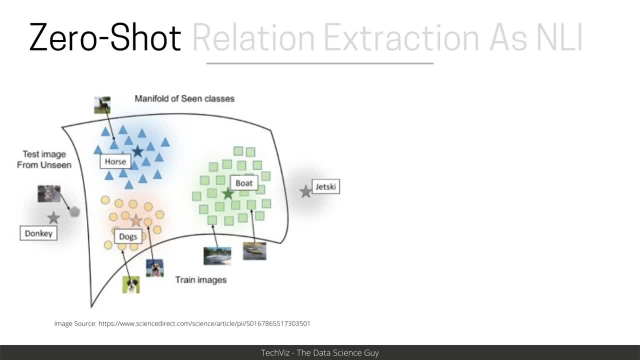 ZSL is expected to also learn and infer to what a donkey would look like. So let's take another example of ZSL that's more relevant in the NLP domain. So let's consider an autoregressive task where you have to predict the next word in the token, given the previous tokens, and we train. 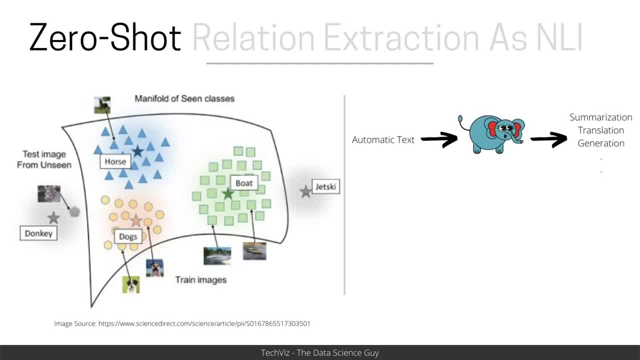 autoregressive models such as GPT-3, GPT-2 and so on. So in this example, if the input text is automatic text, then the next step or the token that the model is supposed to produce should be in the range of, let's say, summarization, translation, generation and so on. So recent results have shown: 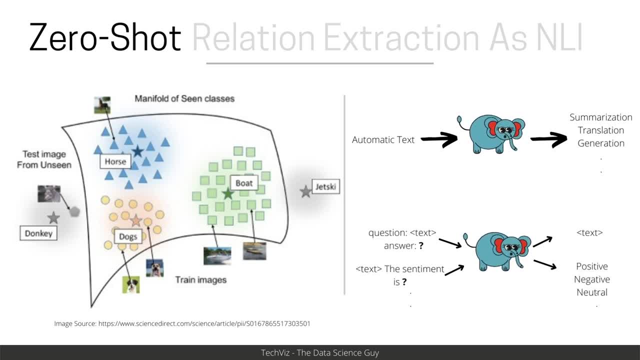 that the autoregressive task of just predicting the next word in the sequence has given these models out-of-the-box capability of making predictions across various tasks. So this wraps up my explanation on ZeroShot. Let's move on to relation extraction. So relation extraction in: 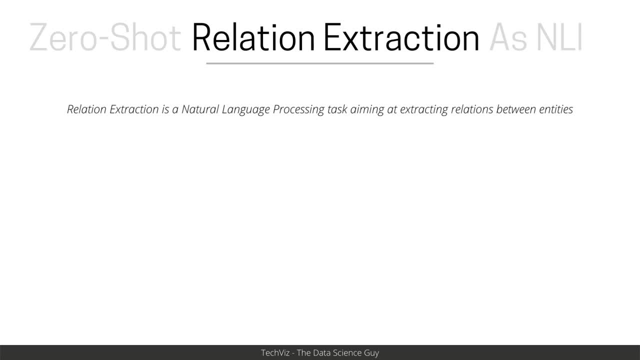 NLP is the task of extracting relation between entities that are present in the text. So let's take an example sentence which is: Barack Obama was born in Hawaii. Now, if we were to extract relation and form triple out of this text, then we could have two versions. Let's say Barack Obama was born. 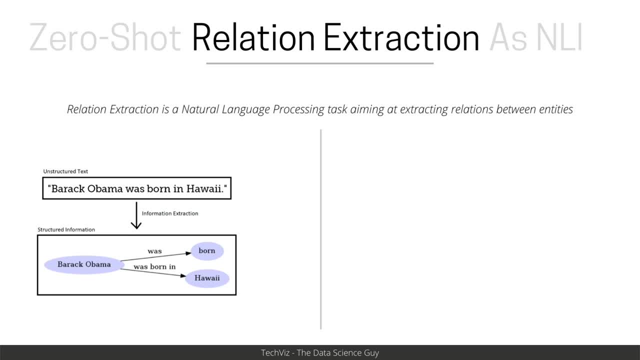 in Hawaii. So unfortunately here it's just the latter makes more sense, but I think you got the idea. Let's take another example from the medical domain and let's say the sentence is: after taking paracetamol, experience nausea. So here the head and tail nodes of a triple would be medicine and 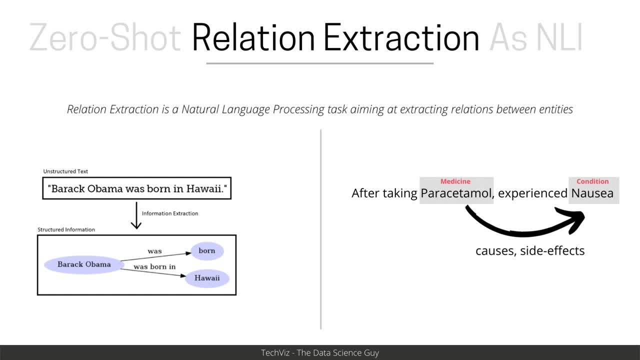 condition and the relation could be cause and side effect. So with these two examples, you must have noticed, in the first example the relation was present in the text itself and that is what we pick it up in extractive sense, Whereas in the second example the exact question is the same. So 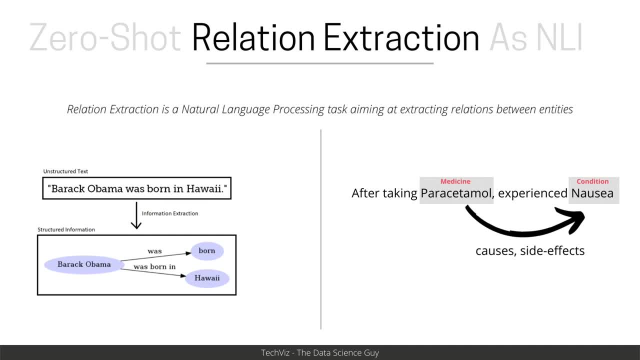 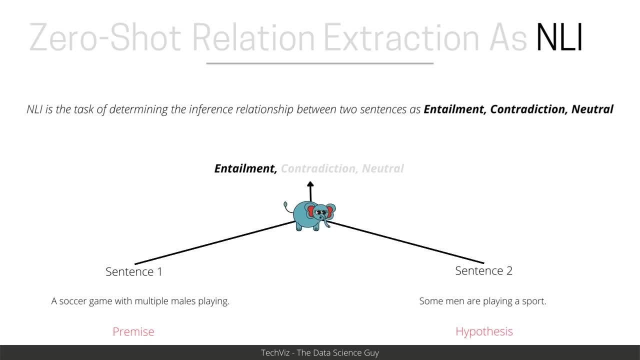 if words were not present, we were able to infer the relation that should go between these two entities. So finally, let's talk about natural language inference task. This is the task of determining the inference relationship between two sentences and categorizing them into entailment. 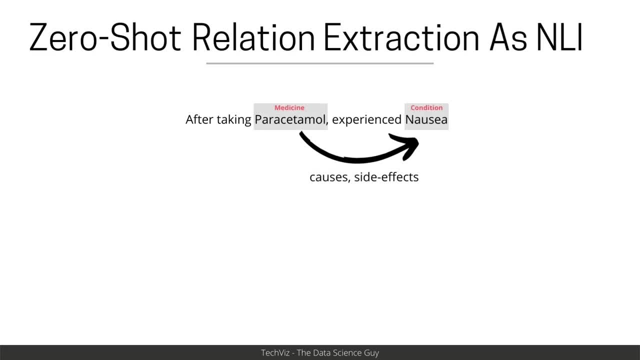 contradiction and neutral categories. So with this we are now ready to join all these pieces and understand what is ZeroShot relation extraction as a natural language inference task. So let's take our old examples from medical domain, where we have our entities as paracetamol and nausea. 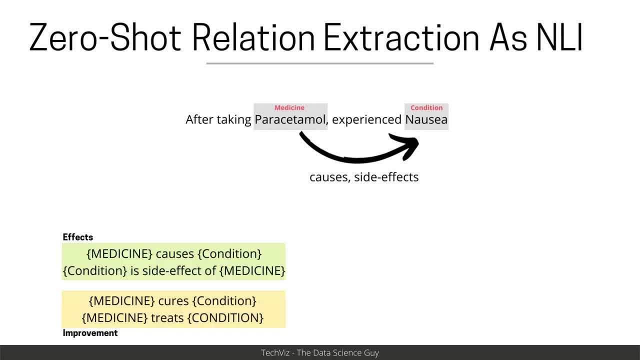 which are tagged as medicine and condition. So, as the first step in the pipeline, once the entities are recognized, we need to form certain prompts or templates where the medicine entities would go in and the condition entities would go in. So, for example, if you define two relation, which is 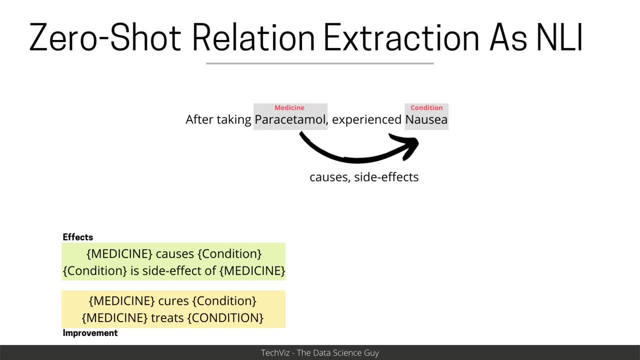 effects and improvement and define certain hand curated and representative sentences that make sense for that relation to hold. The next thing we do is to populate each of these templates and pass on, along with the sentence, to our pre-trained model that is already trained on the natural. 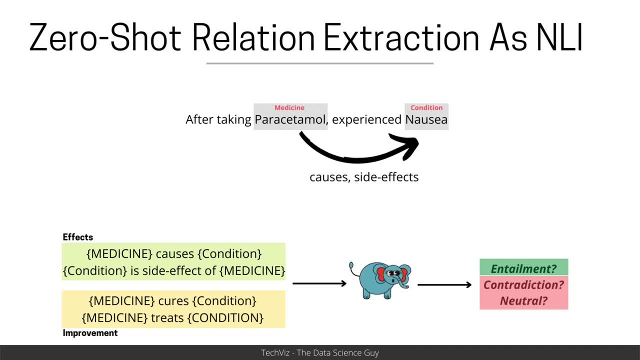 language inference task, which we saw as a part of the previous slide. So here our original sentence would act as a premise and any of the template that we choose from, either effects relation or improvement relation, would act as hypothesis. Now the task of the model is to say if these two 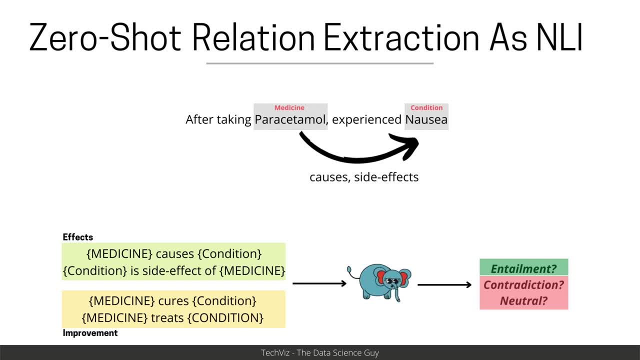 sentences entail or they contradict or they don't hold any relation as such and are neutral. Any prediction made by the model that is not entailment is considered not to hold. So yeah, that's it about how to do ZeroShot for relation extraction as a natural language inference task. But hey, wait a. 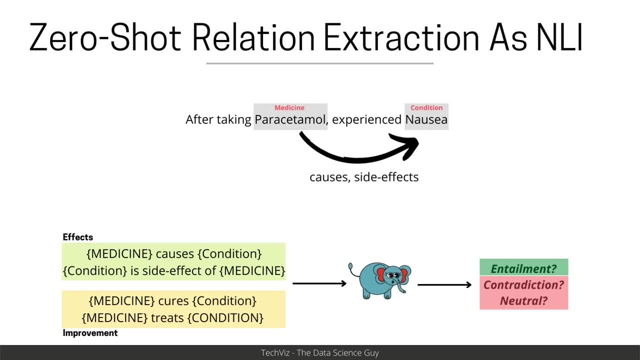 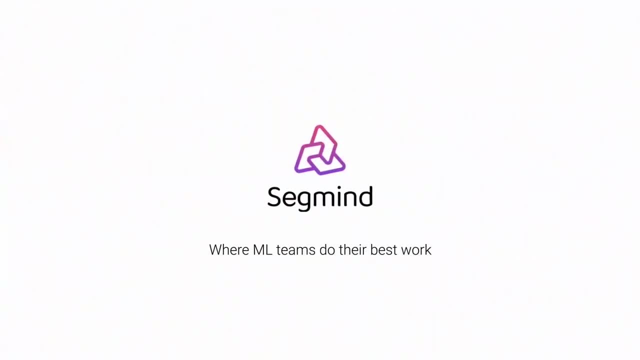 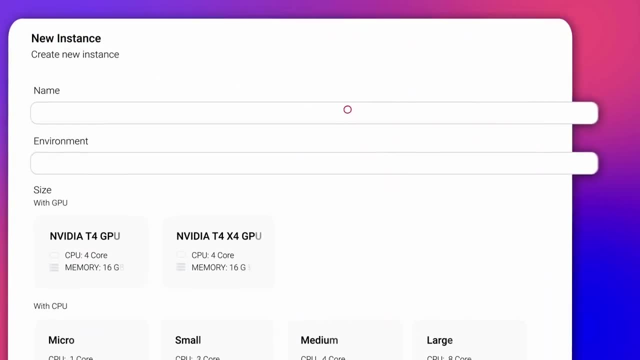 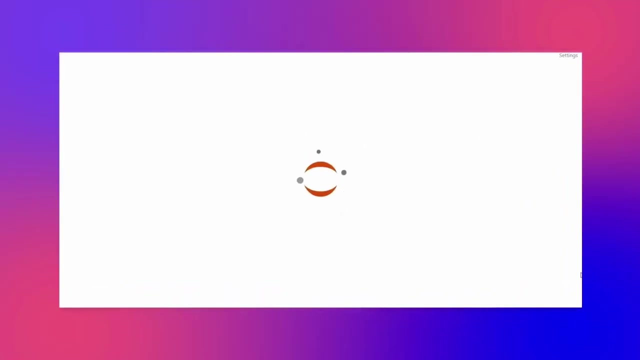 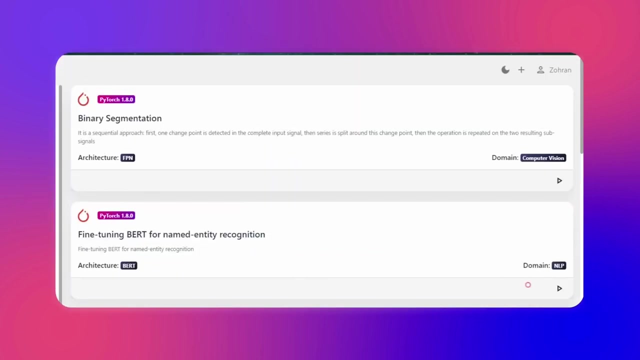 here's a quick overview of what ML developer community can do with this awesome tool, segmine. If you want to learn more about this tool, segmine, you can click on the link in the description to do the sign up and get some free credits. I'll meet you in the next video. Bye for now. Bye, bye and take care.